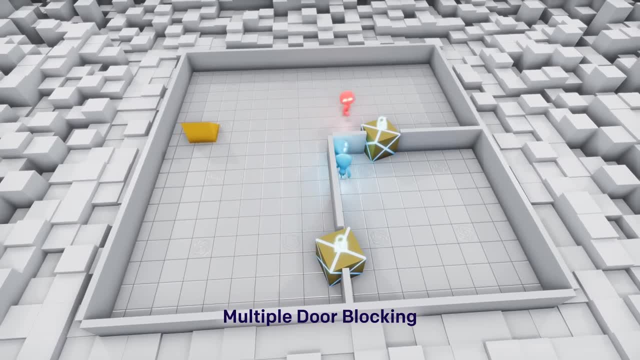 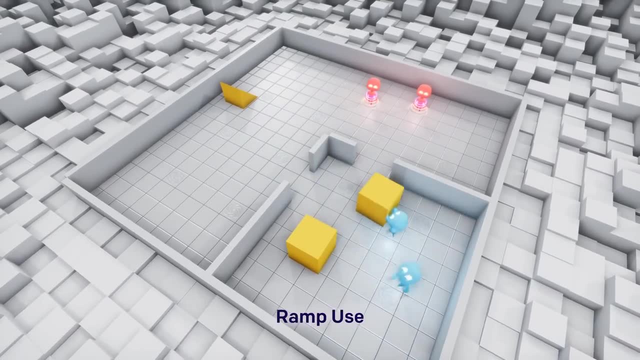 Even so, the hiders must learn to collaborate, accomplishing tasks that would be impossible for any single individual. The hiders are not the only ones who can learn to use tools. After many generations of failing to break into the shelter, the seekers learn to jump over obstacles using ramps. 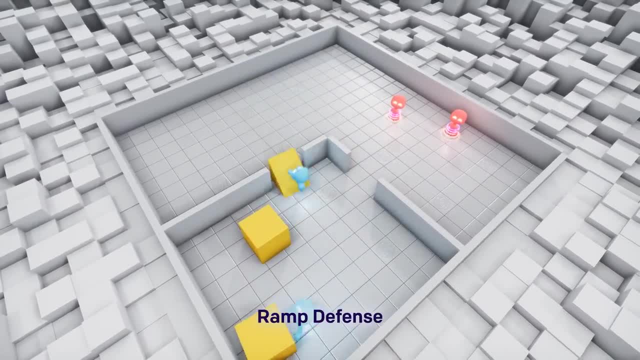 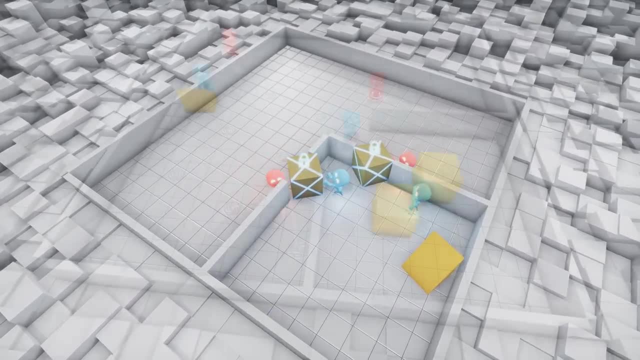 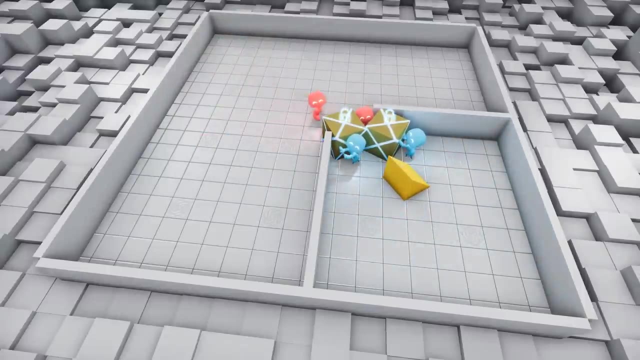 However, after many millions of rounds of having their shelter breached, the hiders learn to take away the primary tool the seekers have at their disposal. Note that we did not explicitly incentivize any of these behaviors. As each team learns a new skill, it implicitly changes the challenges the other team faces, creating a new pressure to adapt. 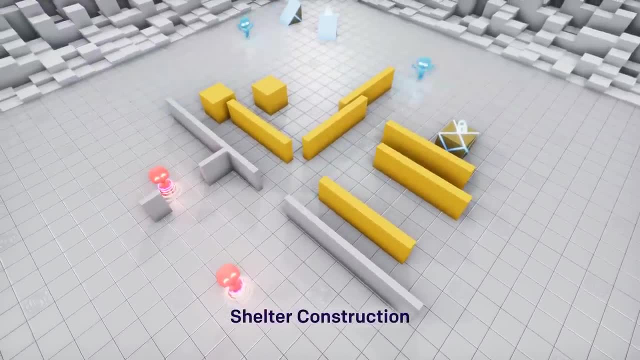 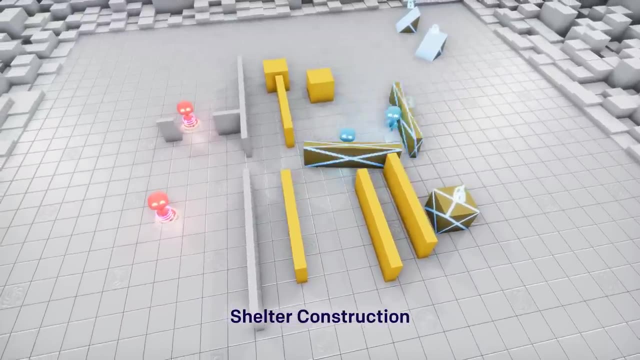 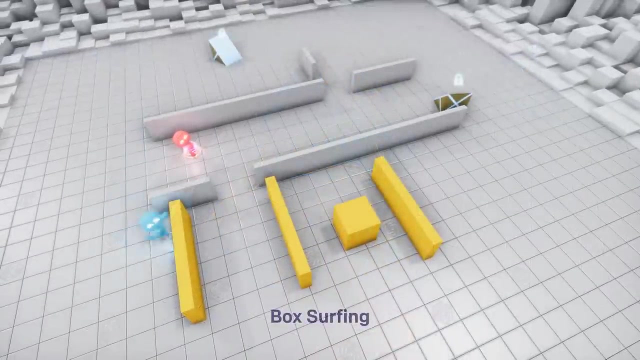 We've also put these agents into a more open-ended environment, randomizing the objects, team sizes and walls. In this world, they learn to construct their own shelter from scratch, requiring that they arrange multiple objects into precise structures To prevent seekers from using the ramps, the hiders, move them to the edge of the play area and lock them in place. 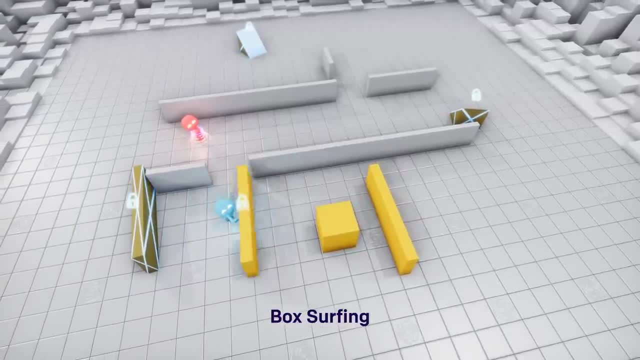 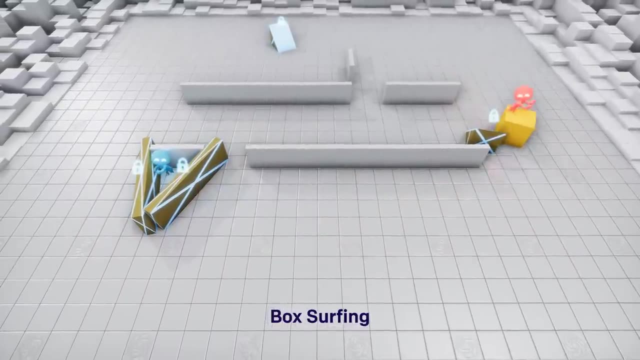 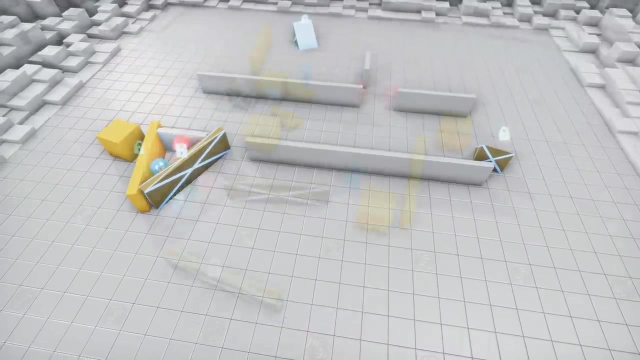 We originally believed this would be the final strategy that the agents learn. However, we found that after more training, the seekers discover that they can jump on top of boxes and surf them to the hiders' shelter In the last stage of emergent strategy that we observed. 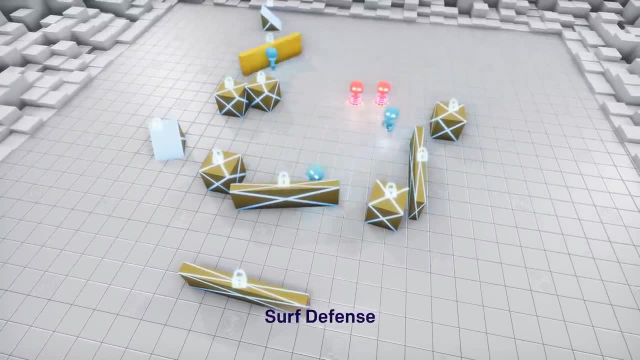 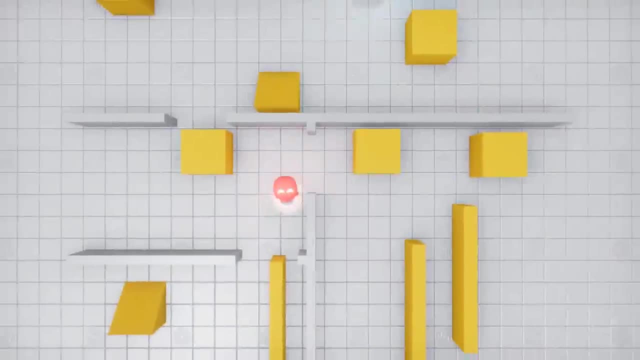 the hiders learn to lock as many boxes as they can before constructing their fort in order to defend against box-surfing. So how do agents acquire these skills? They're trained using reinforcement learning, an algorithm inspired by the way animals on Earth learn. 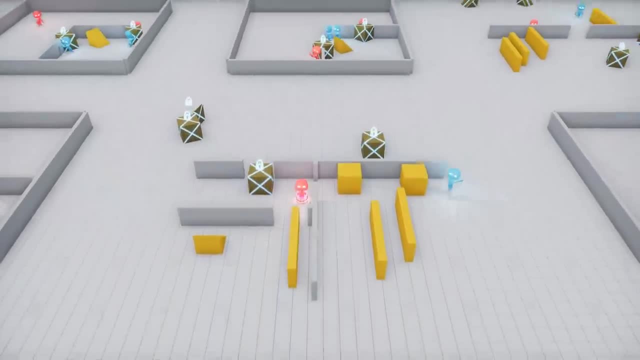 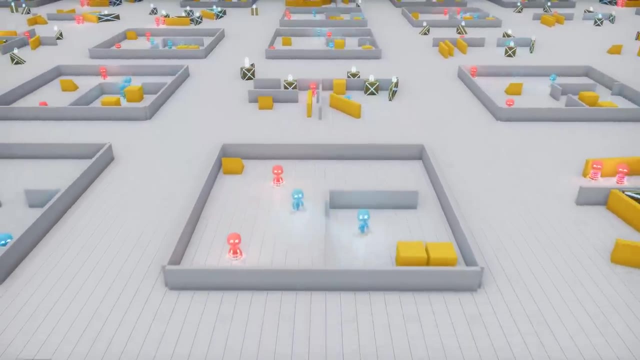 The agents play thousands of rounds of hide-and-seek in parallel for many days. They train against each other as well as past versions of themselves, using an algorithm called self-play. Co-evolution and competition on Earth led to the only generally intelligent species known to date: humans. 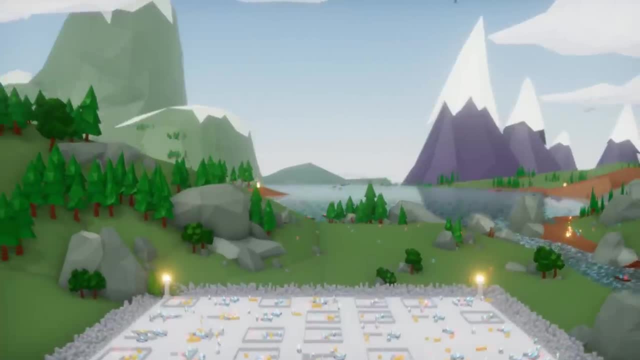 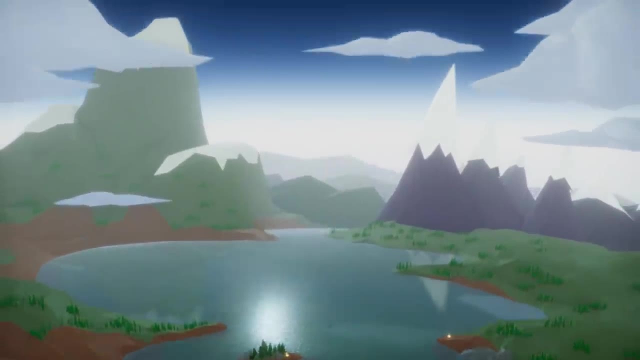 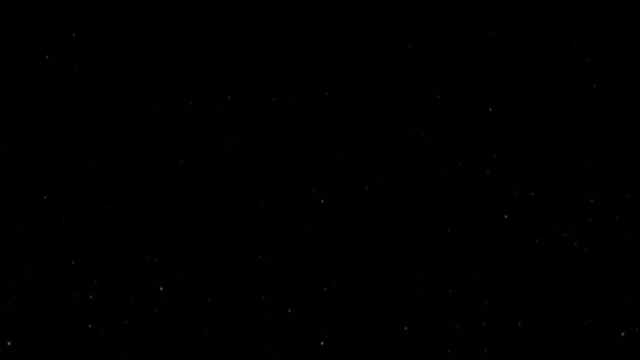 While this world is far less complex than Earth, we have found evidence that simple rules can lead to increasingly intelligent behavior from multi-agent interaction. We hope that with a much larger and more diverse environment, truly complex and intelligent agents will one day emerge.